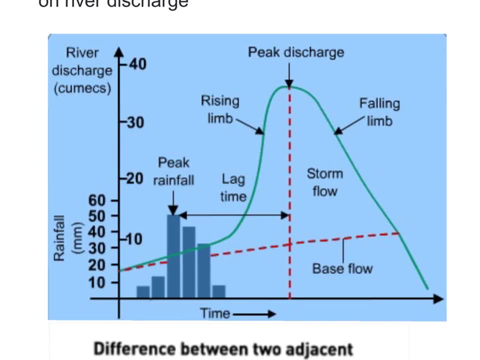 following labels which you would need to understand to be able to answer an examination question on this. The x-axis on a storm hydrograph will always have time as its label, and this can vary in terms of hours- it could be days or it could be months, just depending on the exam question that you get The y-axis. 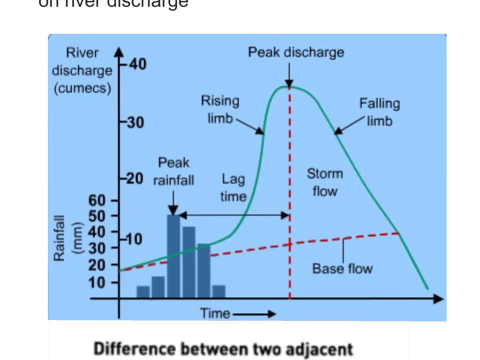 will normally have two different labels. in this case we can see river discharge, which is labeled here, and we also have rainfall, which is labeled here. Most, if not all, storm hydrographs will show the precipitation event. so you can see here, from these number of bars of this bar graph, that we have a storm event. 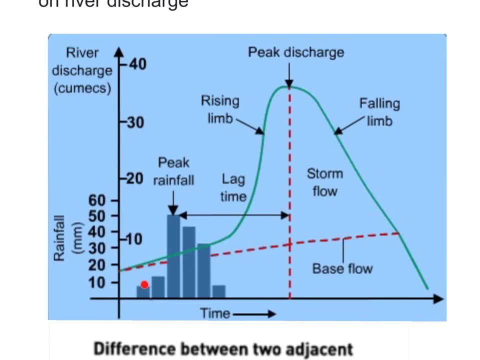 happening in this drainage basin. So for each time period here you can see the volume of precipitation and again, that's important- Over to the line graph aspect of this, which is really the, the hydrograph that we want to talk about. Basically, this is showing the impact that this 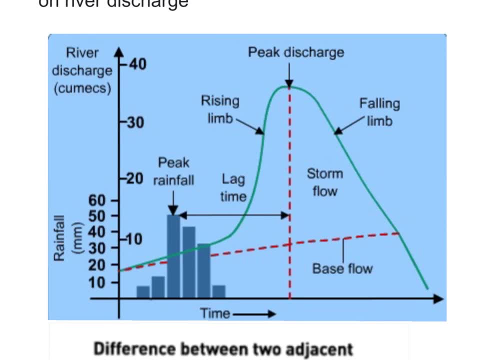 event or precipitation event has on river discharge in this drainage basin. The response to any precipitation event will be different for different drainage basins because those drainage basins all have different characteristics. Some of the general points that you need to know or labels that you need to understand: 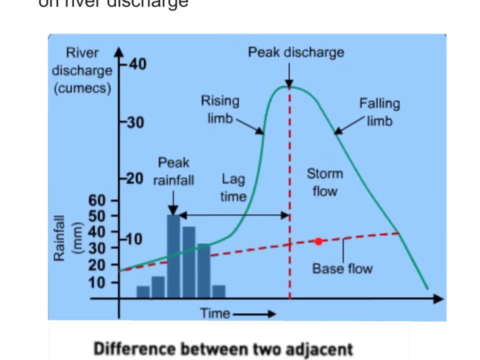 about the drainage basin. First of all, we have this line which is labeled base flow. this is basically the general normal flow without any impact of precipitation on the river, so just the normal flow of a river or the normal discharge in the river. This next section, anywhere above this line, is referred to. 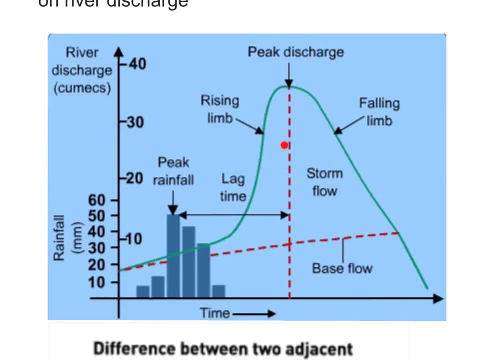 as storm flow. so any flow in this area is in response to this precipitation event. This green line up to here is referred to storm flow. This green line up to here is referred to. This green line up to here is referred to as the rising limb, and after it's reached its peak, it's referred to as the falling limb. 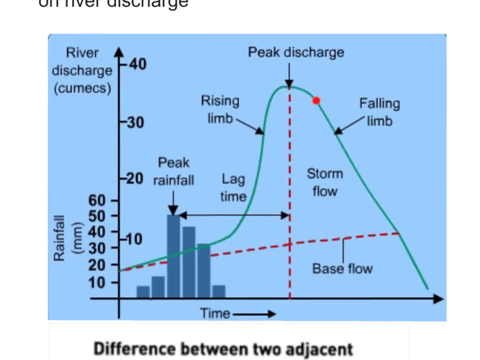 This will rise in relation to the precipitation event and then it will fall after the precipitation event has ended. This is referred to as peak rainfall and this is referred to as peak discharge. Obviously, peak rainfall is the maximum amount of rainfall. This is the maximum amount of discharge in the river. 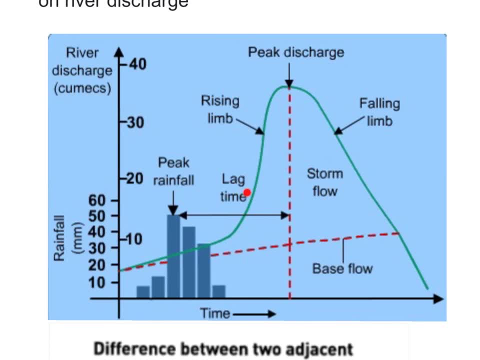 The difference between these two times is referred to as lag time. Lag time again will be different for different drainage basins. So that's the overview. maybe, if you haven't quite grasped all those terms, it might be useful to rewind the video and have another look at it. 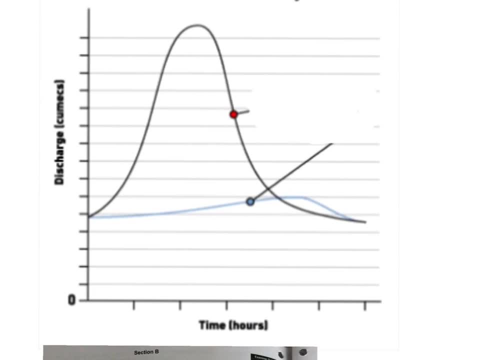 In terms of thinking about hydrograph. here's a slightly different graph. We don't have a precipitation event on this. This is really just to illustrate how you need to get this clear in your head. There are two real extremes of hydrographs. 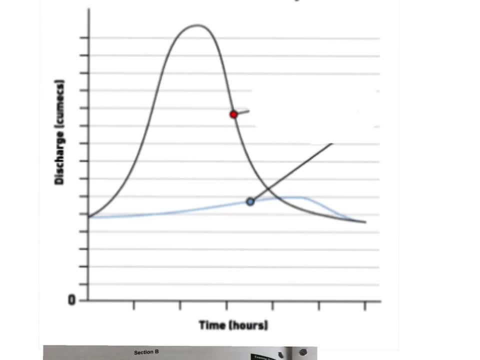 This line refers to discharge which is similar to the one that we've just had and we call that a flashy hydrograph response. And that flashy response has a number of characteristics, So you can see here that it has a very steep rising limb. it has a very high peak discharge. 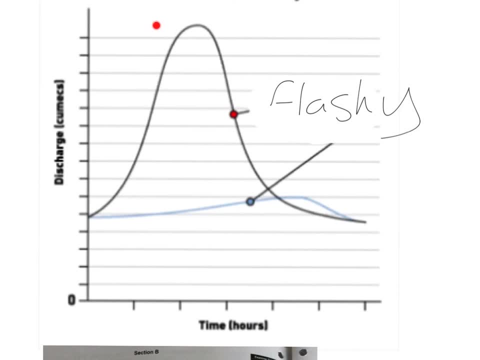 and if we could see lag time, it would be so This is a very giant discharge. It's a very, very light discharge. have a very short lag time. The other extreme is represented by the blue line and it's referred to as a flat hydrograph, And once again, flat hydrographs. 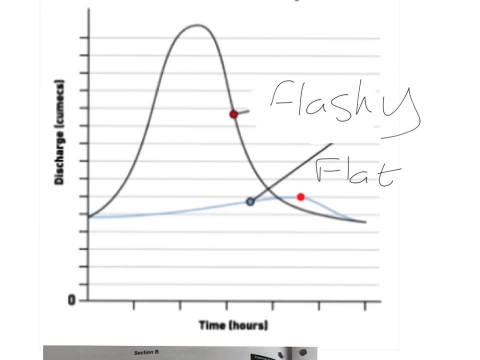 have certain characteristics: They have a low peak discharge, they have a gentle rising limb, they have a gentle falling limb and they have a very long lag time, which we can't see on this diagram. So that's what you need to think about with regards. 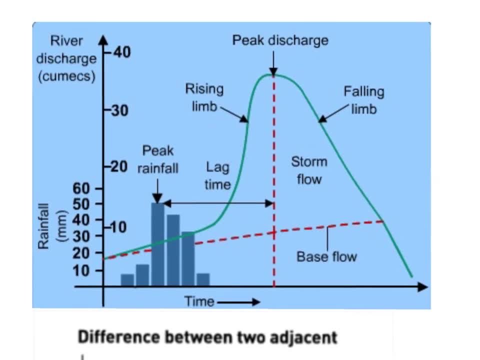 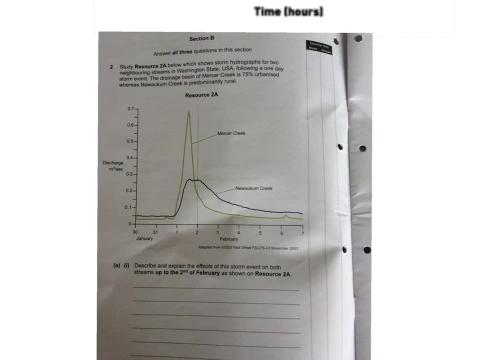 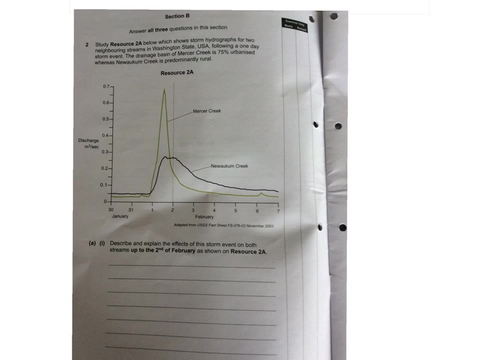 to preparing for the exam. There are the overview of the labels and there are your two extremes- flashy and flat- and their characteristics. Here's your likely exam question. So again we can see storm hydrograph here. Remember what I said to you, that we get time along the bottom In this case.